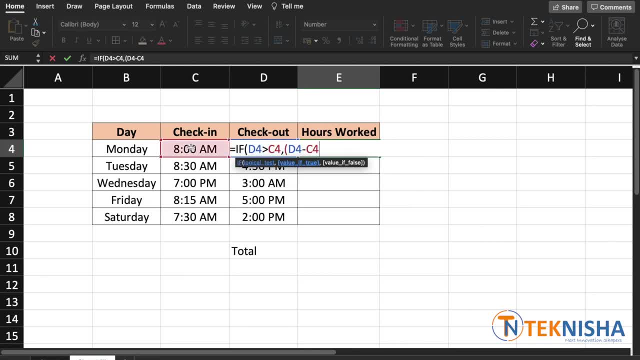 which is d4 minus c4. else, if d4 is less than c4, then we go with d4 minus c4 plus 1, which basically adds 24 hours, and the output of this, if condition, needs to be multiplied by 24, so we get: 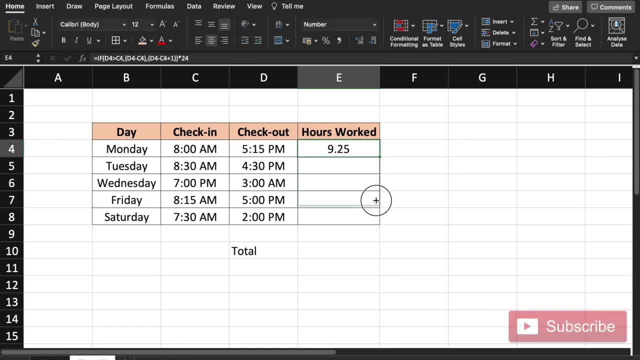 nine point two: five on Monday, eight hours on Tuesday and eight hours on Wednesday also. so now doing the total is really simple. all we need to do is put in the formula equal to sum of the range e4 to e8- you, so I'm just going to format this. so let's say, if you now change this time, 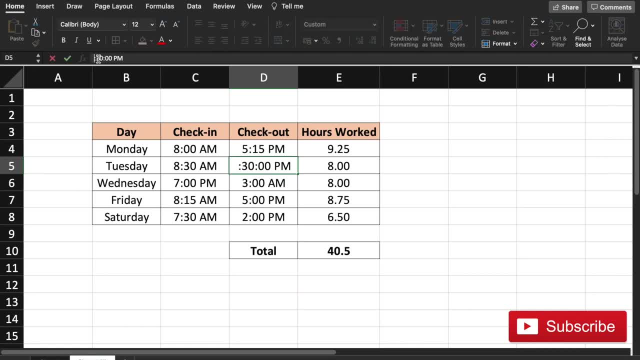 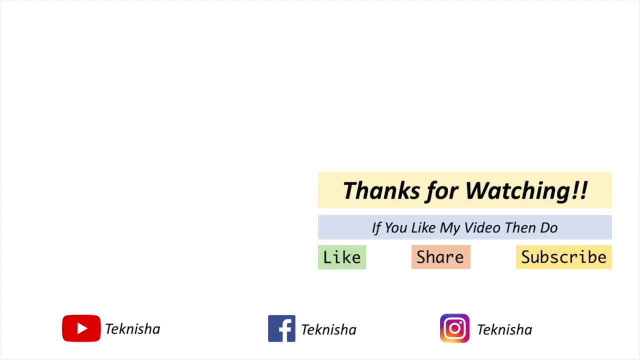 from 430 pm to 530 pm. you get nine hours and then the total is updated. I hope that this tutorial was of use to you. if you liked it, please subscribe to my channel till next time you. 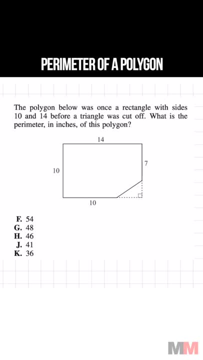 The polygon below was once a rectangle with sides 10 and 14, before a triangle was cut off. What is the perimeter in inches of this polygon? In order to find the perimeter, which is the distance around, we have to find this little piece that's missing right here, and if you focus on that shape, it is. 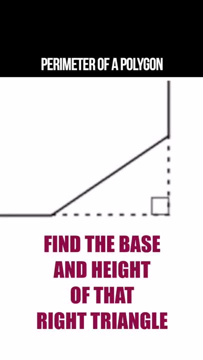 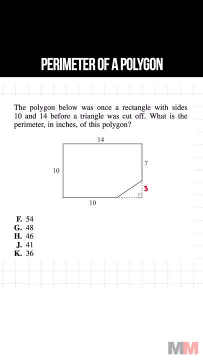 just a right triangle. So first let's find the base and height of that triangle. We can find the height by just taking 10 minus 7, and that's going to equal 3.. Doing the same strategy for the base: just take 14 minus 10 and we will get this base right here, which equals 4.. On these tests, 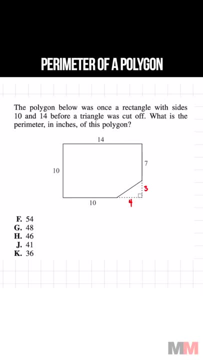 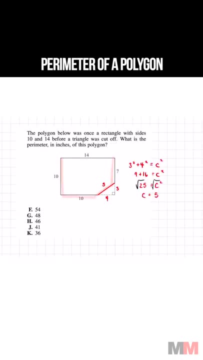 they love to use the 3, 4, 5 triangle. You could have noticed that this missing piece right here was 5, or you could run through the Pythagorean theorem. And now that we got that measurement, then we just got to add all the dimensions around the shape, which is going to equal 46. letter choice.